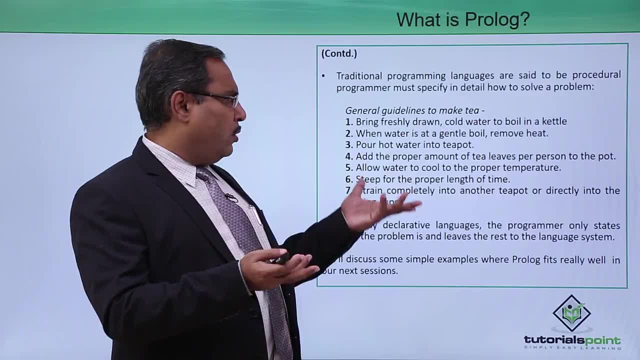 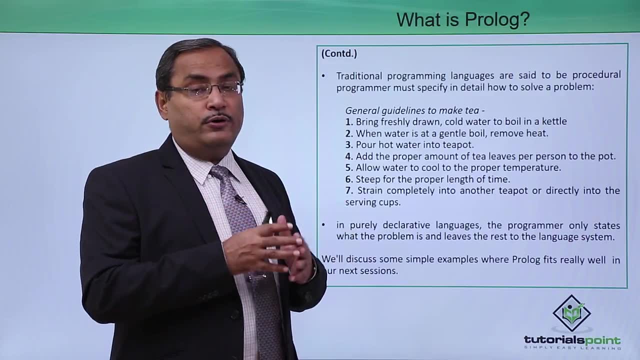 So it will be defined by the procedural programming language. Just consider general guidelines: to make a tea, a cup of tea, if you want to make a cup of teas, So for your guests. so, obviously, what are the steps you are supposed to follow? So, step number one: take some. 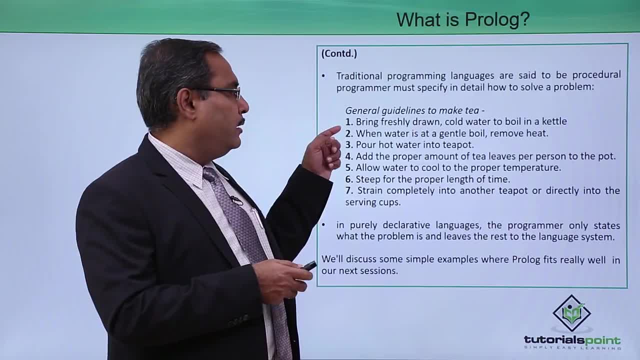 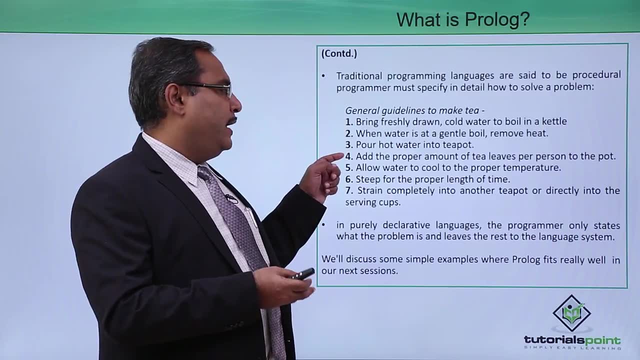 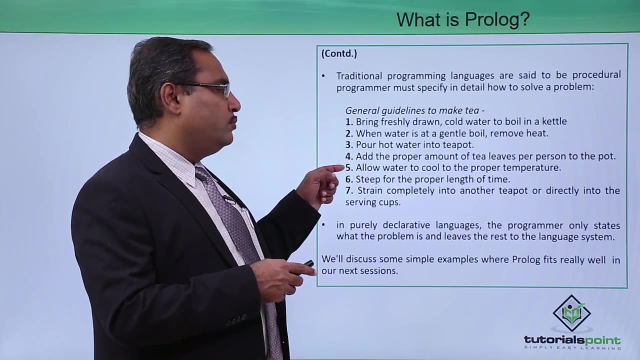 fresh water and boil it in a kettle. Then, when the water is at a gentle boil, remove heat. pour the water onto the teapot. add some tea leaves and some sugar on it, or you can add sugar later on. also, Allow water to cool down to proper temperature. steep for. 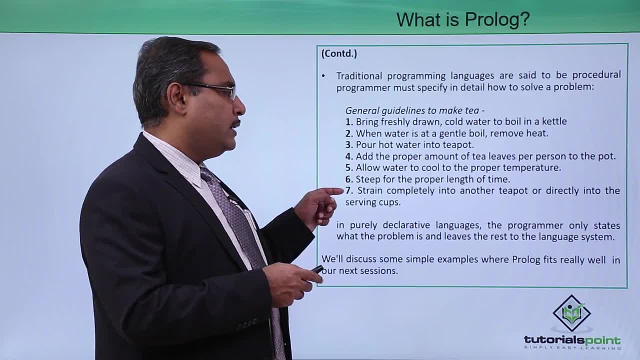 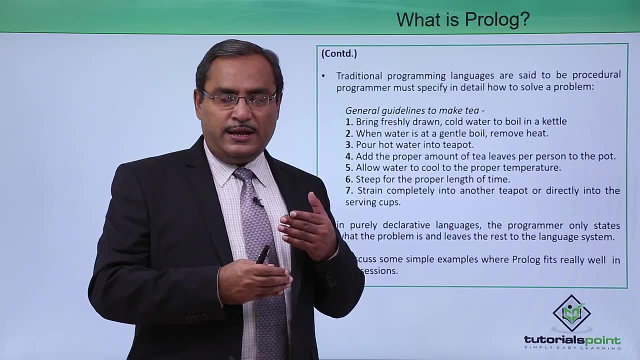 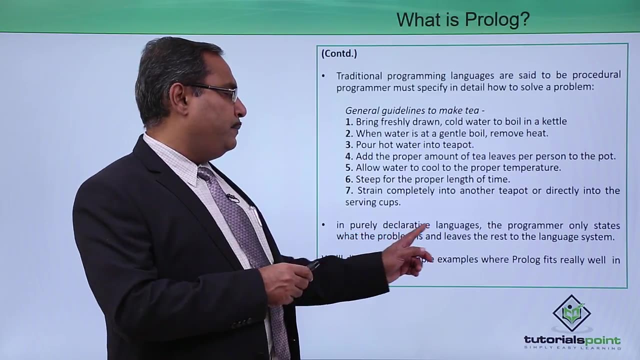 the proper length of time, strain completely into another teapot or directly into the serving cups, and you can add sugar after that also. So these are the steps required. So these are the steps required And this is very much analogous with these procedural languages In purely declarative. 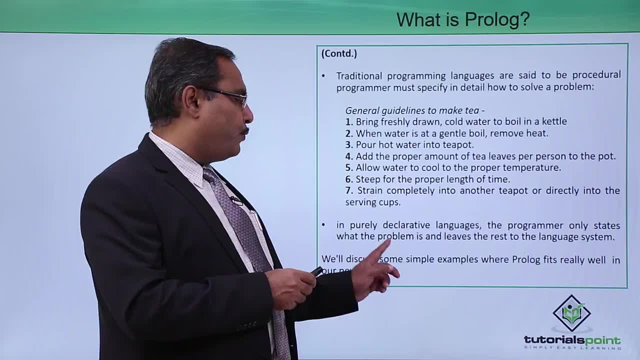 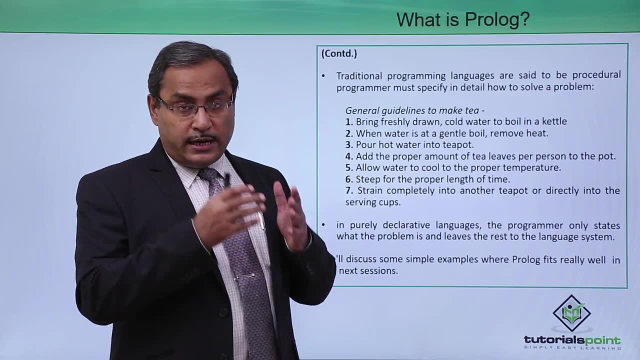 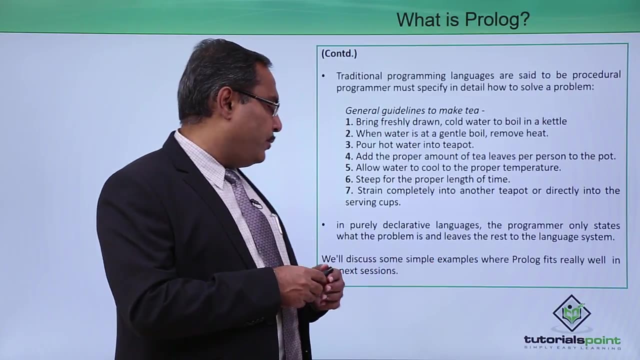 languages. the programmer only states what the problem is and then leaves the rest to the language system to derive whether how to get the required output. We will discuss some more simple examples where Prologue fits really well in our next different video sessions. So please watch the video. 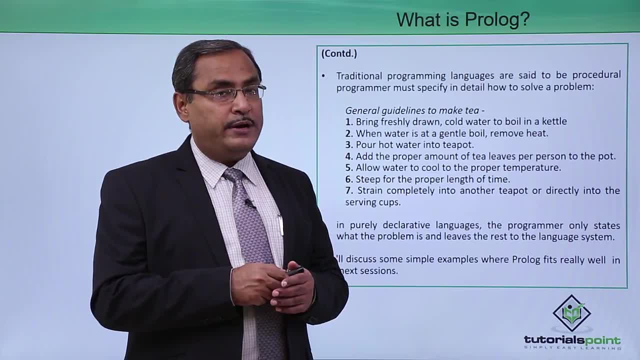 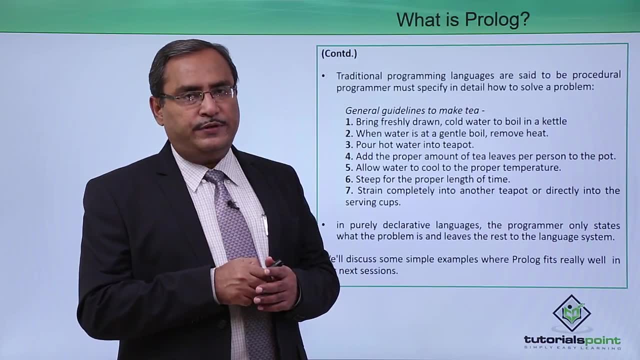 Watch all the videos where we will be discussing how the Prologue programs can be written and what are the different issues involved with this Prologue programming. Thanks for watching this video.